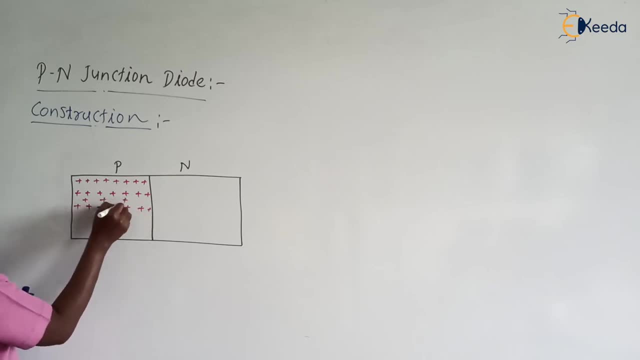 and a small number of negative charges are present in the p type material. so suppose a small number of negative charges are present in the p type material, okay, so in the construction of pn junction we are having the pn type material. okay, so next, whereas the n type material consists of large number of negative charges. 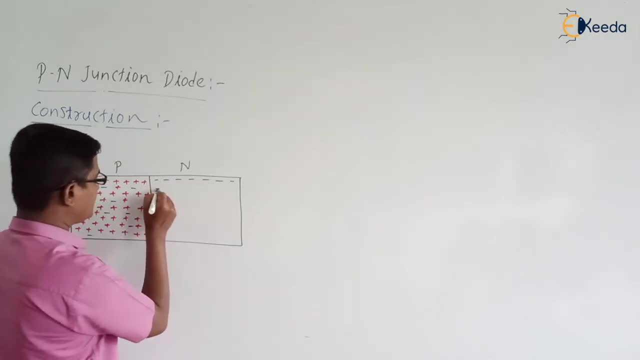 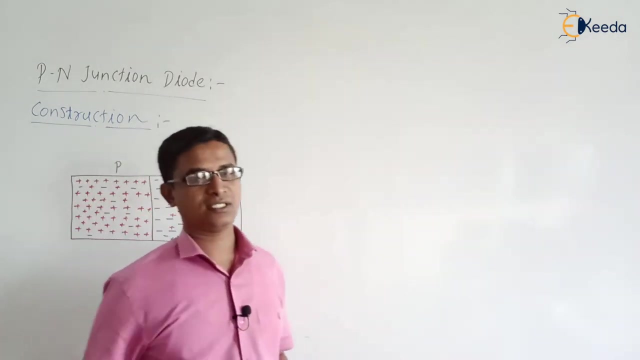 so we are having very large number of negative charges present in the n type material, and the n type material consists of large number of negative charges and the n type material consists of very small number of positive charges. okay, so this is the pn junction. okay, why it is a known as pn junction? because it consists of p type. 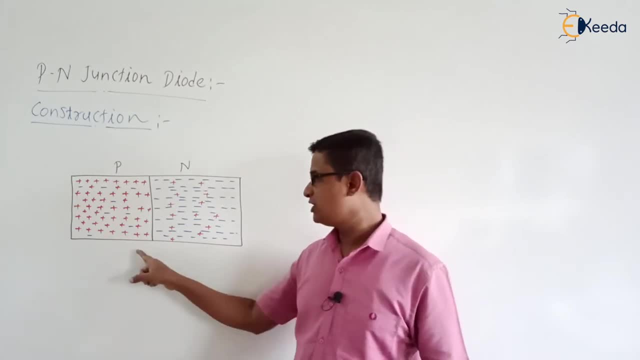 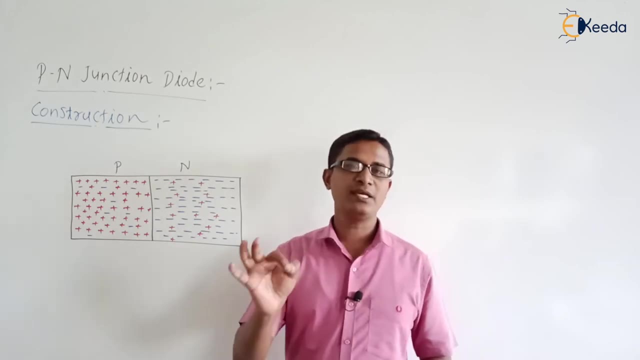 material. it consists of n type material and in between these two, here we are having the junction okay. here we are having the junction okay of the two layers, so that's why it is known as the pn junction okay. so now we are having the two different materials at one side. large number: 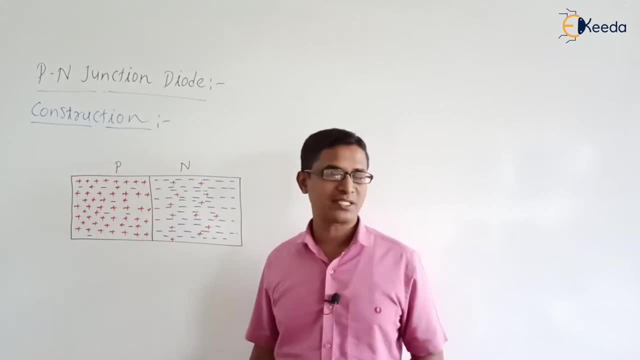 of positive charge carriers are there and very small number of negative charge carriers are there. at the second side, large number of negative charge carriers are there and very small number of positive charge carriers are there. okay, so can we say that the density of the density of positive 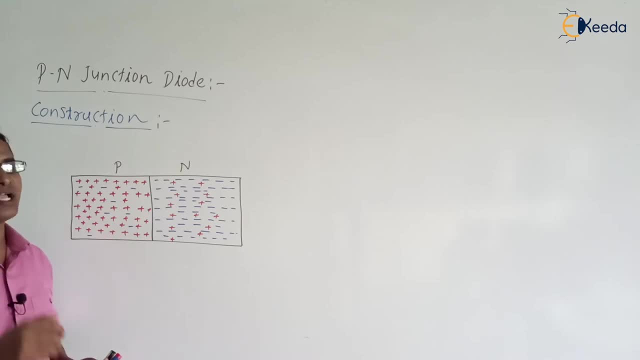 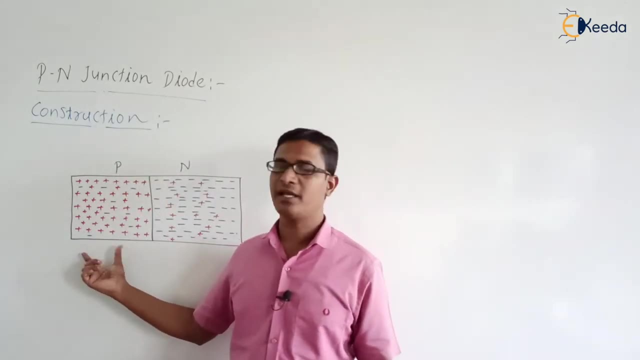 charges in the p type material is very, very high. what do you mean by the density? density is nothing but the number of charges right divided by the volume of that layer. okay, so if we want to find the density of the positive charges in the p type layer okay, then we can say that the number of 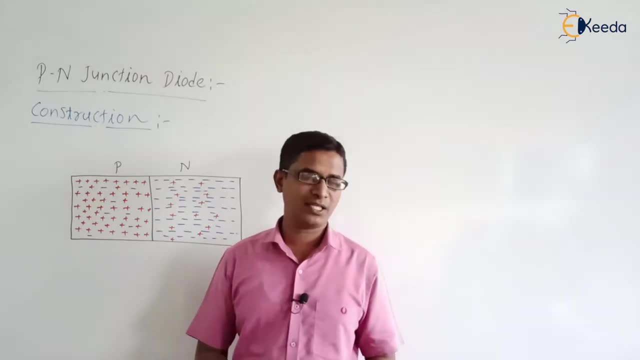 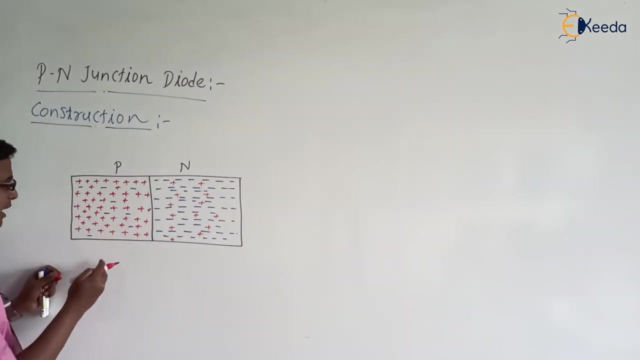 positive charges which are present in the p type layer, or the p type material divided by what is the total volume of that p type material or the total area of the p type material we can see. okay, so that will give you the density. okay, so here we can write the p type. 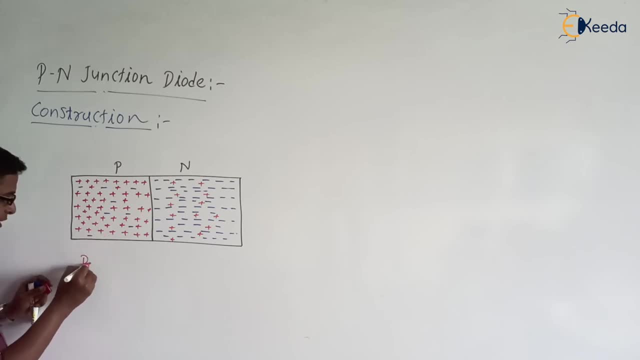 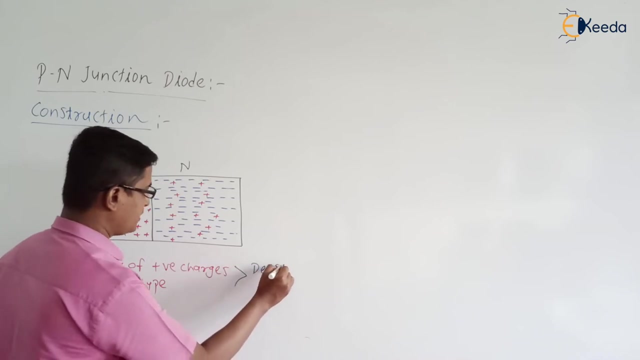 material consists of large number of positive charges. so density of positive charges, density of positive charges in p type, in p type material, is greater than density of negative charges. sorry. density of is greater than density of positive charges in n type material. okay, so the density of positive charges here is greater than. 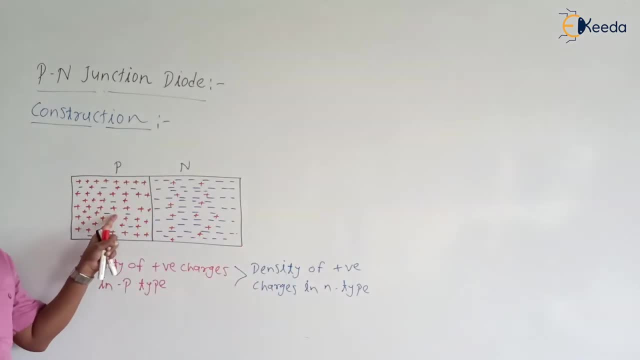 that of the density of positive charges here. okay. similarly, can we write: the density of negative charges in the p type is less than the density of negative charges in the n type. okay, so we can write: density of negative charges is less than ча ntyp. so if we try to calculate density of positiveừng, 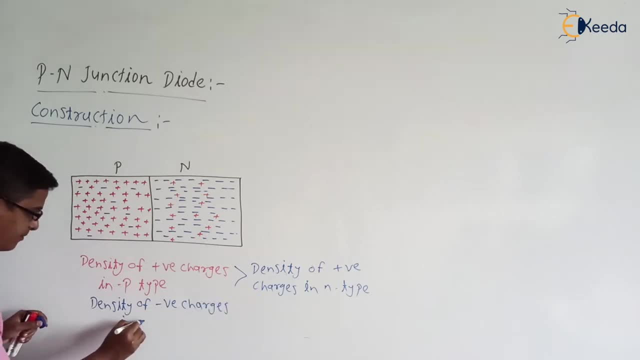 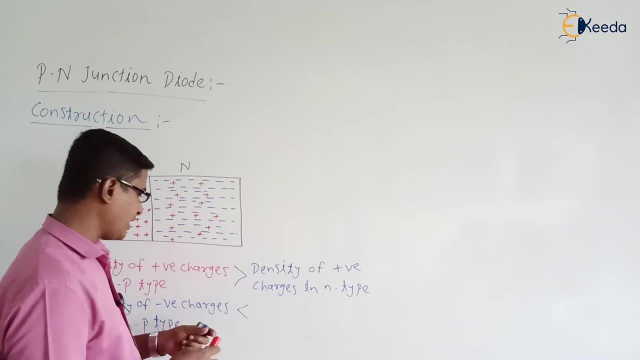 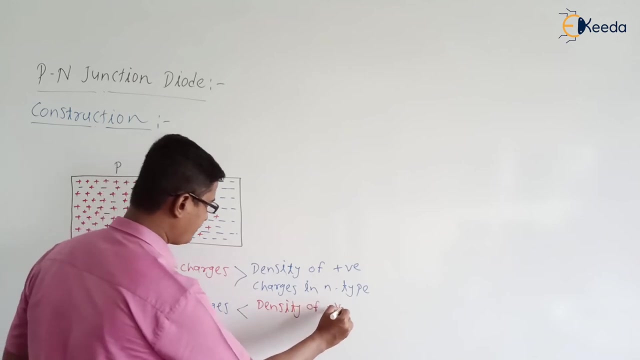 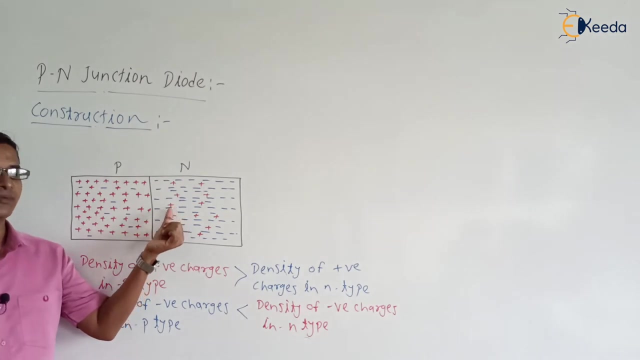 in p type. density of negative charges in p type is less than density of negative charges in n type is less than density of negative charges in n type- material. okay, so here we are having the density of positive charges more here. density of positive charges very less here. 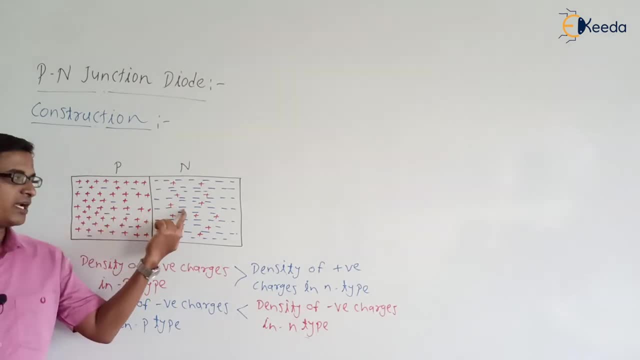 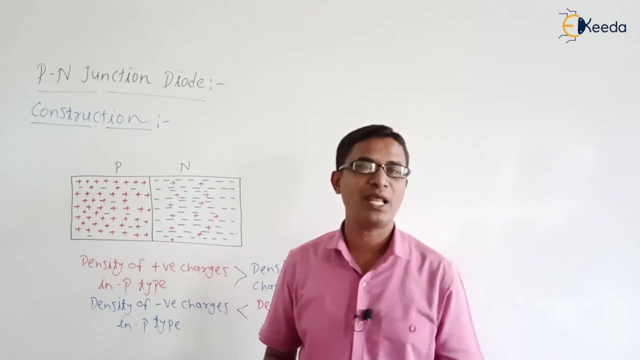 density of negative charges: very less here. density of negative charges: very high here. okay, so, these are the materials we are having and now we are connecting these two materials. okay, so what will happen as soon as these two materials are connected together, as soon as these two metals? 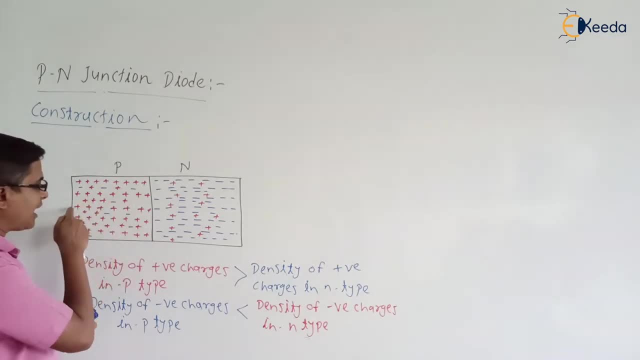 are connected together. so what will happen? as here we are having the large number of positive charges and here we are having the very small number of positive charges. so what will happen? the positive charges from p type material will try to cross the junction and will try to move towards the n type material. 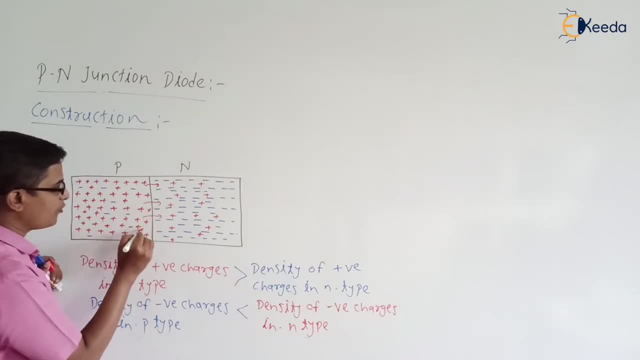 okay, so from here to here the positive charges will be moving from p to the n type material. okay. similarly, here the density of negative charges is high and the density of negative charges in the p type material is very, very less. okay, so as soon as these two layers are, 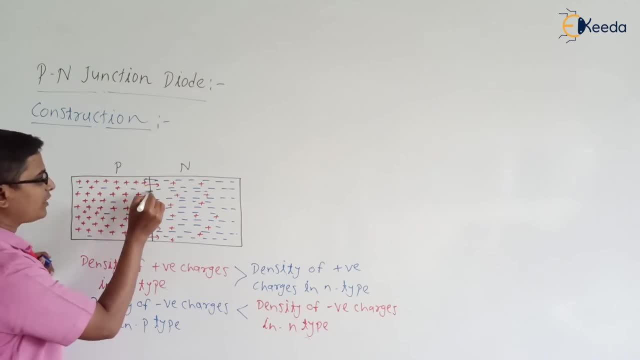 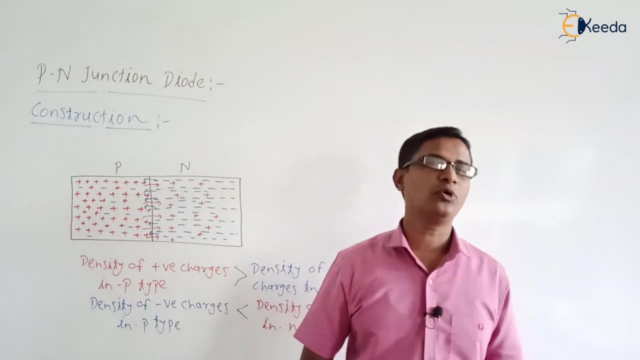 connected together, the negative charges from n type will try to cross the junction and will try to enter into the p type material. are you getting the point? okay? so here negative charges will be moving from n type to p type and the positive charges will be moving from p type to n type. now, as soon as now, as soon. 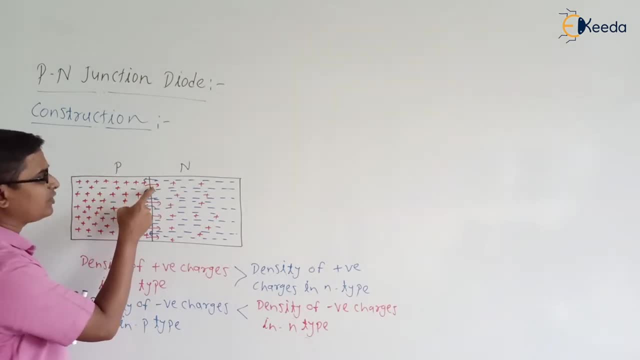 as yes, the suppose this positive charge will enter into the n type material. okay, so, first of all, this positive charge. where, at which position, at which, at which place this positive charge will occupy its place? yes, definitely it will occupy its place. okay, so here the positive charge will rotate declinately to the right. here, yes, and here over here, see. 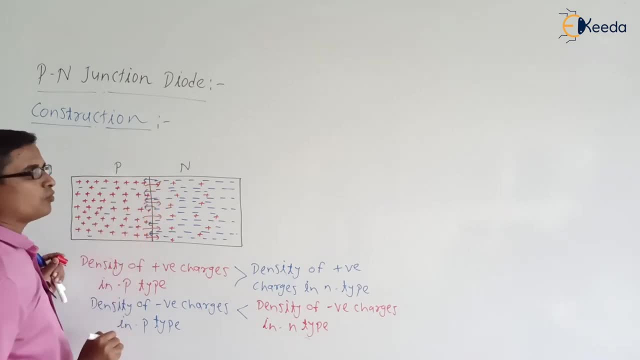 that this, vamos positive charge will move from p to the location. that's why this pure, this positive flow of this positive flow is very, very n type, material right. so these positive charges from p to n type will charge the space of the patient and it will naturally de feet. 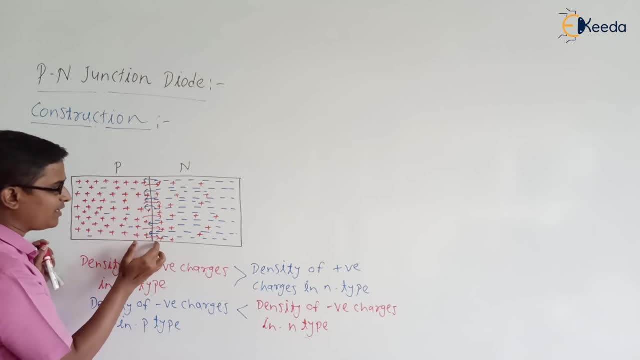 also. yes, wither removed me. this is the n type and it is inside the compound. so we have to re下來, touch this side, this side, we will a and then we have to bring the new data. so what is the exact will occur after crossing the junction? this positive charge will accumulate. 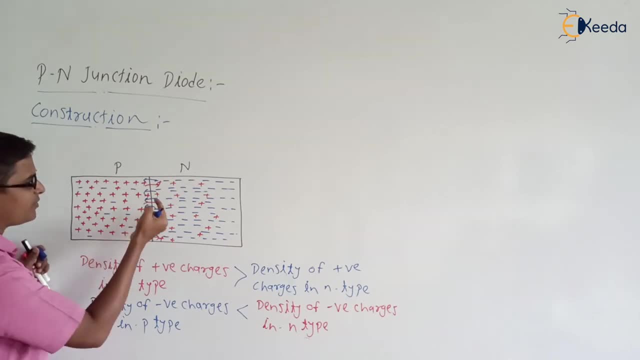 the space at this position only, or near to the junction only. okay means whatever the positive, When the negative charges are coming from n-type to p-type, these negative charges will try to occupy the space. will try to occupy the place near to the junction, only okay. 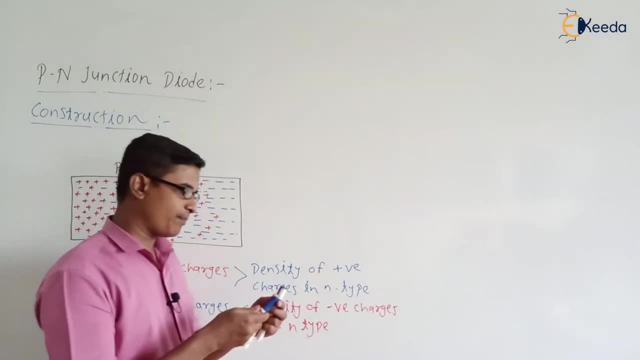 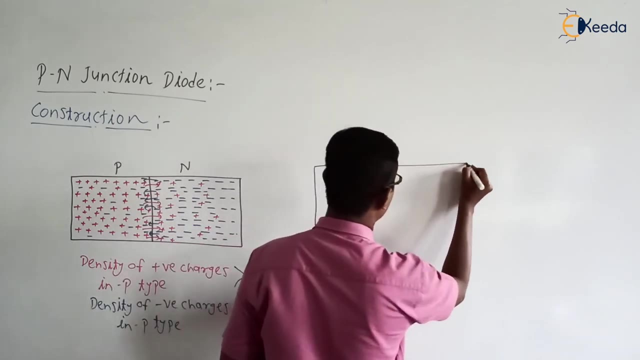 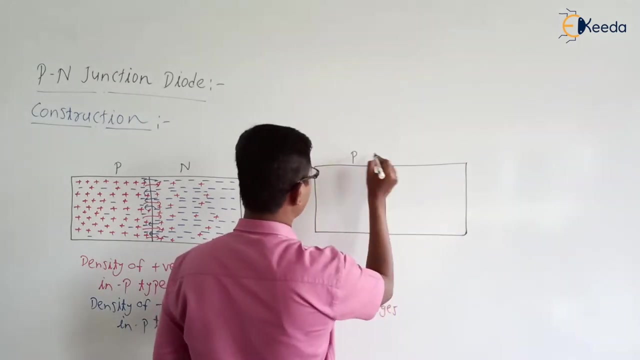 So if you check after connection of the p-type and n-type material, we will be having one type of the layer near to the junction right. So once p-type and n-type materials are connected together here- suppose this is p-type, n-type- at the p-side we are having a layer of negative charges which is formed near to the junction. 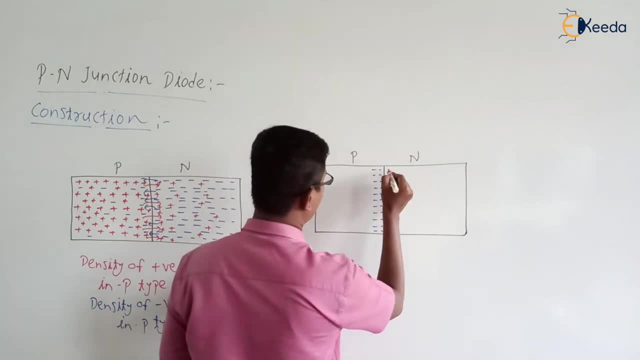 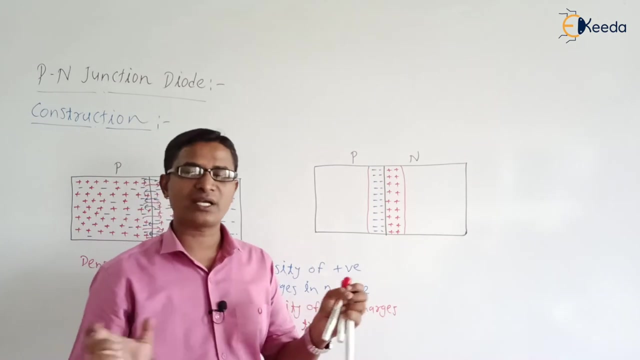 And at n-type, we will be having a layer of positive charges which is formed near to the junction. So this is p-type, So this is p-type, So this is the layer which is present near to the junction. okay, So, as soon as we connect the p-type and n-type material, okay, then what will happen? 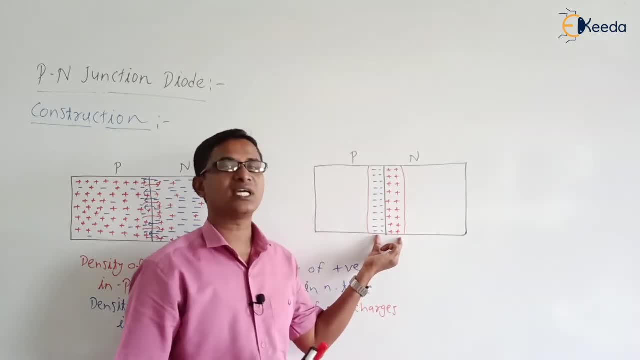 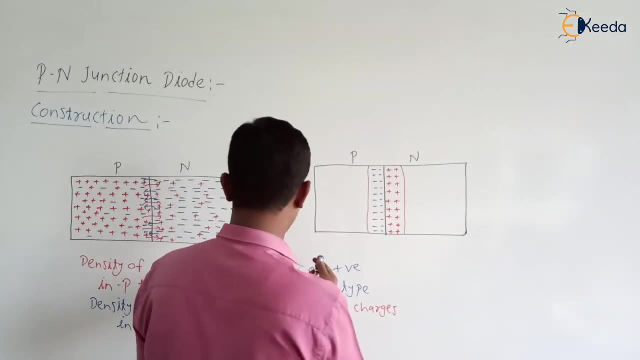 Here we will be having one layer near to the junction and that layer is known as the depletion layer. That layer is known as the depletion layer. okay, Of course, here in the p-type we will be having the large number of positive charges, as it is. 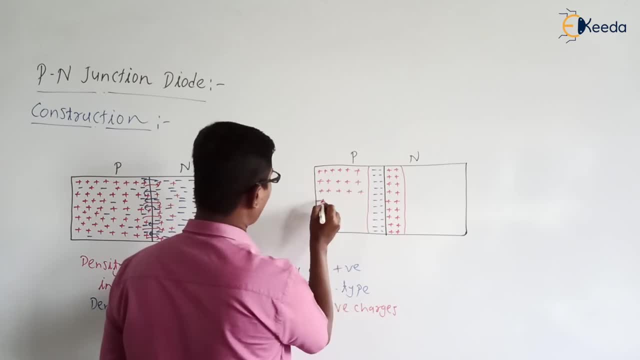 But some positive charges will move from p-type to the n-type And they will occupy the space near to the junction right. So, similarly, here we are having the small number of negative charges that will be present. okay, Next here, large number of negative charges. as it is, 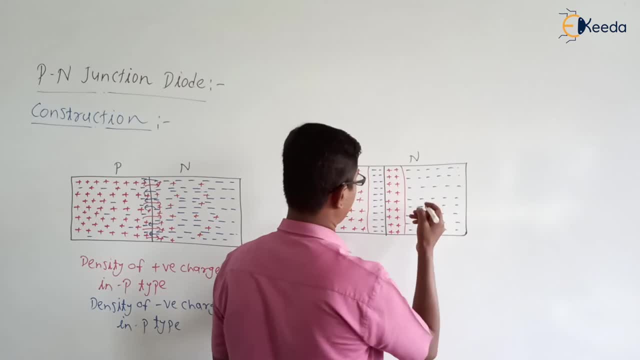 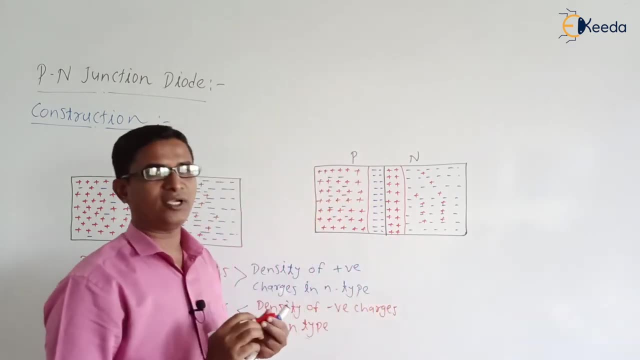 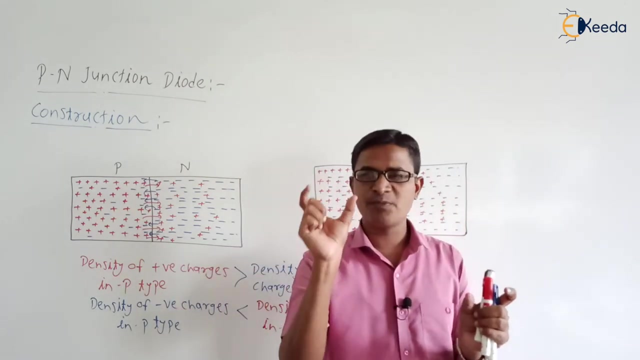 Okay, And small number of positive charges And small number of positive charges Right. Are you getting the point, Okay, Why this depletion layer is formed? Because we have connected the two layers. We have connected the two materials: One is a p-type, second one is a n-type. 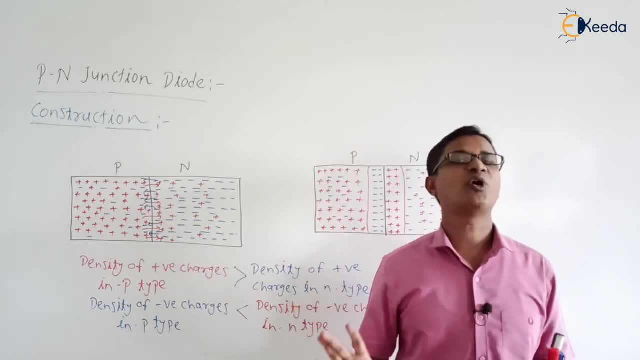 In the p-type, we are having the large number of positive charges and very small number of negative charges. In the n-type, we are having the large number of negative charges and very small number of positive charges. So as soon as these two layers are connected together, definitely the positive charges from p-type will be formed. 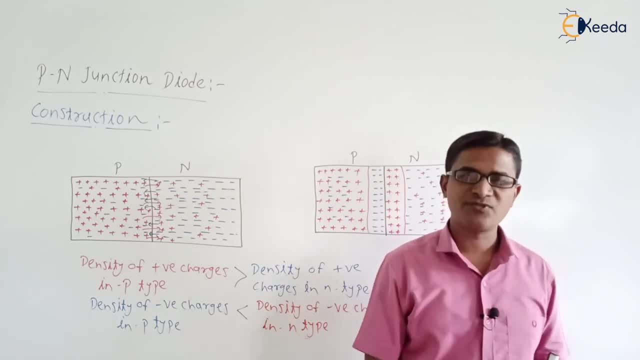 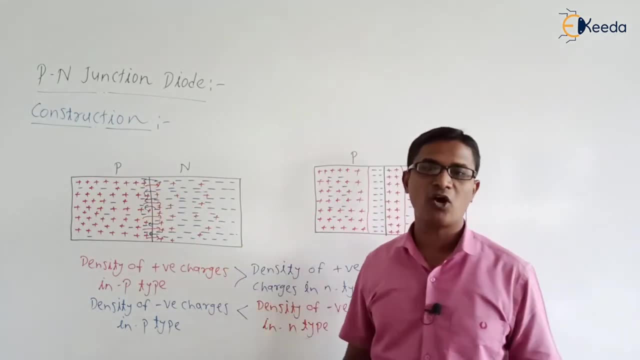 And the negative charges from p-type will try to move towards the n-type And the negative charges from n-type will try to move towards the p-type. okay, But after moving or after movement? yes, these charges will occupy the space near to the junction only. 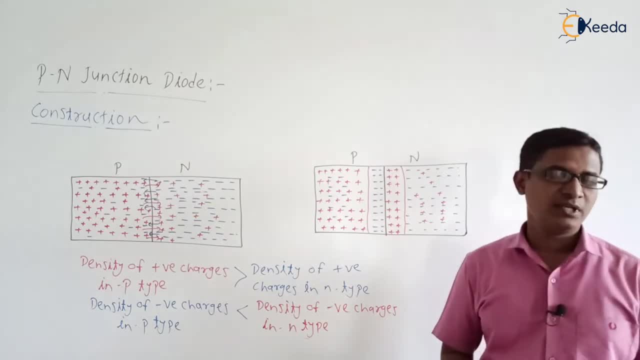 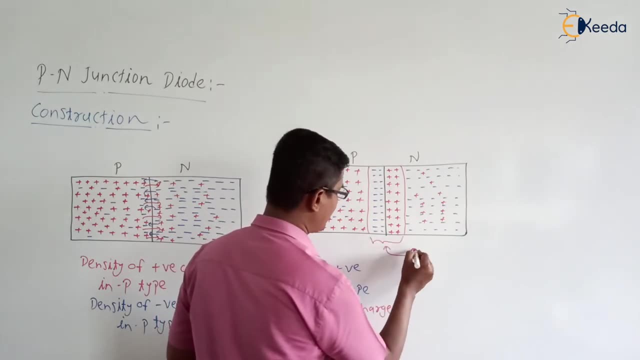 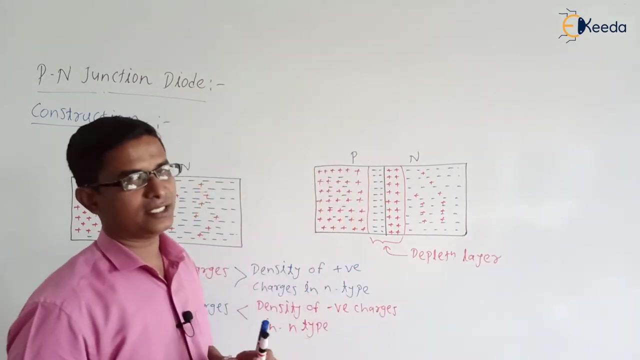 And it will cause the formation of one layer near to the junction, okay, And that layer is known as the depletion layer. This layer is known as depletion layer. Are you getting the point? Okay, So this is the depletion layer. Are you getting the point? 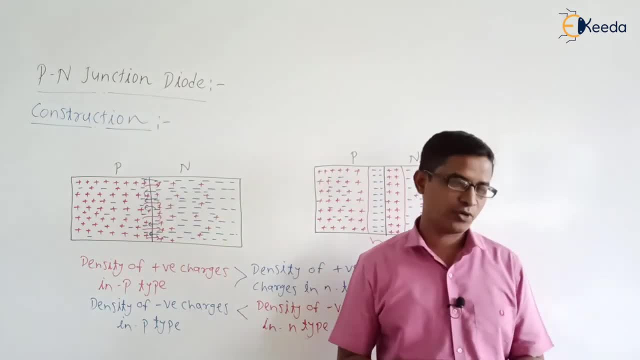 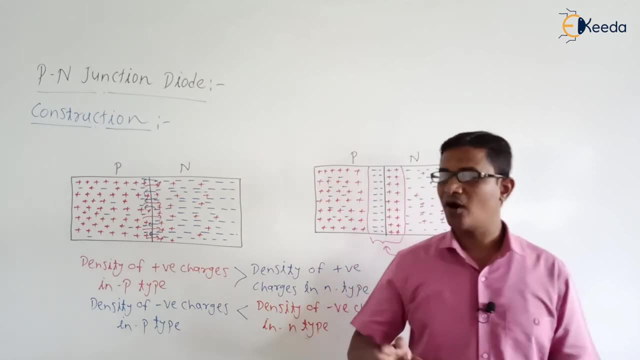 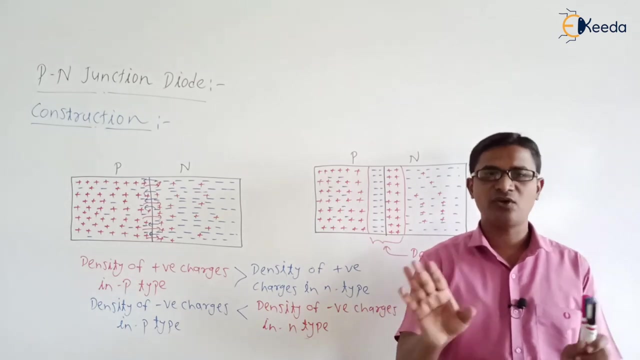 Okay. So suppose if we go into the market and if we purchase the diode, okay, By default in that diode there will be, yes, the existence of the depletion layer. okay For the formation of depletion layer, whether we have applied any external source, we have connected any external source across the diode. no,